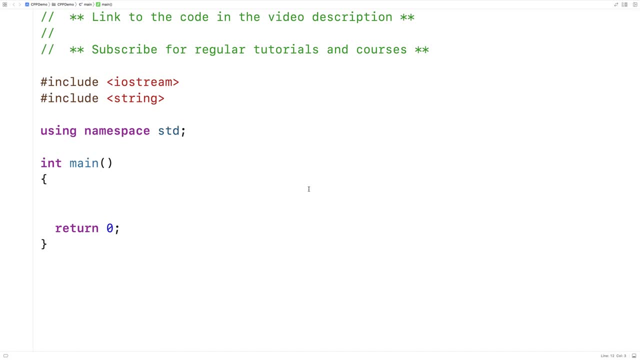 Let's say that we want to write a computer program to work with banking Accounts. If you think about your bank account, there's many pieces of information that are associated with it, So, for example, your name, the balance in the account. 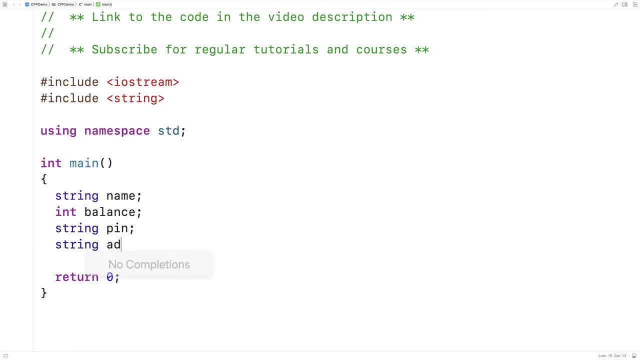 the pin for the account, the address for the account and perhaps the unique ID for the account, like the bank number, And there's probably many more pieces of information associated with the account. Now, already working with this many variables all separate is going to be kind of a mess. 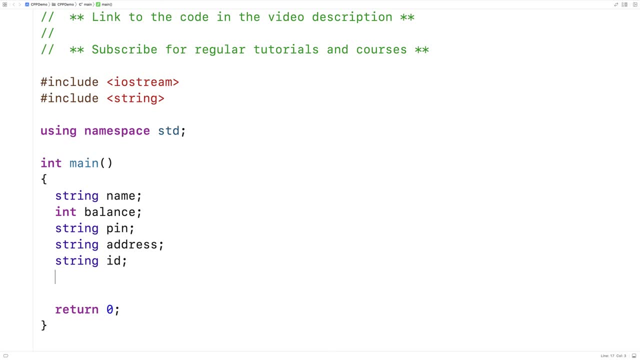 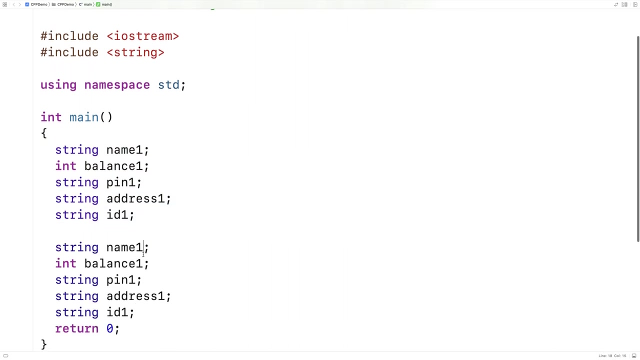 Imagine, though, we need to work with multiple or many bank accounts. We could start trying to number the variables. We could say: name one, balance one, pin one, address one, ID one for the first bank account, And then maybe say: name two, balance two, pin two, address two, ID two. 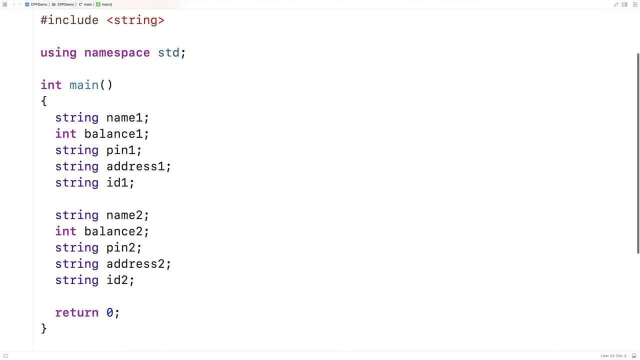 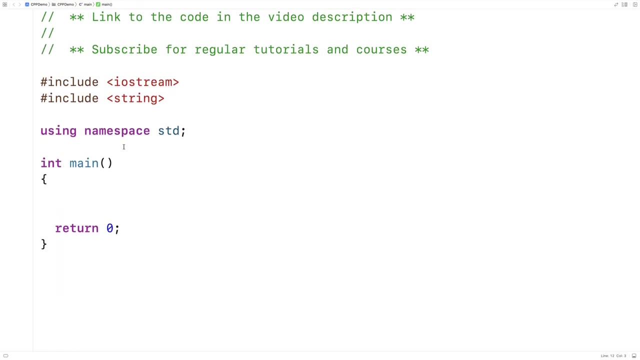 for the second account, We could even try creating a series of arrays for each chunk of information. But no matter what we do, this is going to be a messy way of working with the data. What we really need is a way to define a new type of thing that has these sorts of fields of. 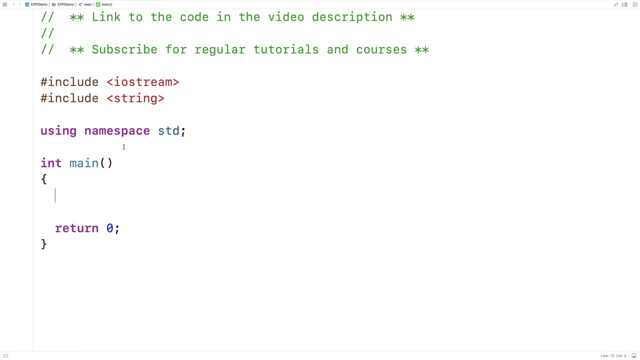 information as sort of properties of that thing, because a bank account just fundamentally has more than one chunk of information associated with it. So we can create what's called a class, which is a type of user-defined type. So here we'll say class: bank account. 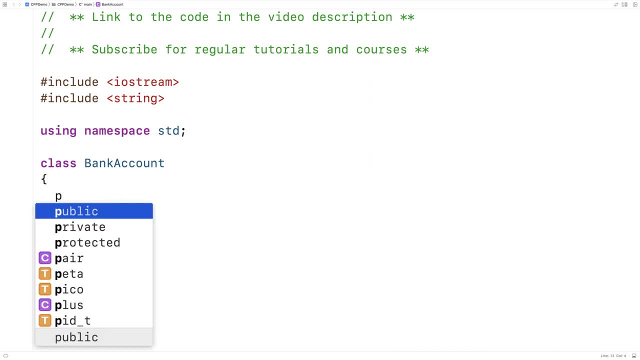 open squiggly, close squiggly. We'll put a semicolon here And then we'll say public, colon, string, name and int balance. So what we've defined here is a new type of thing, a new type of object called bank account. 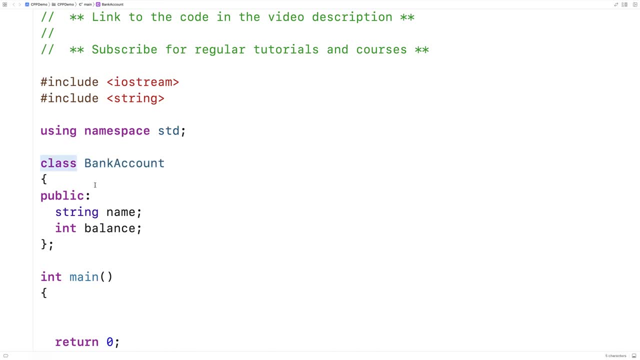 And we're using the class keyword to do this. We could say that bank account is a class, It's a type of object. Here we're defining two member variables, two members of this class: the string name and the int balance. Now, this public keyword here is what's called an access specifier And the public access specifier. 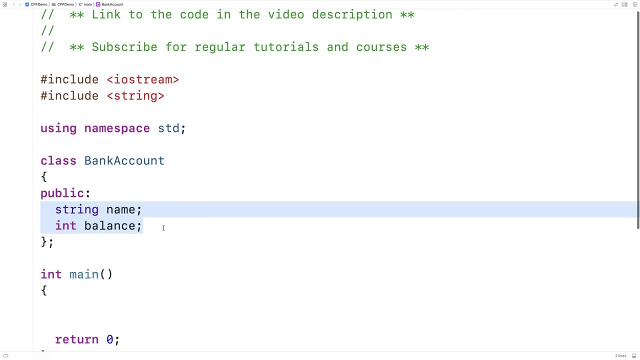 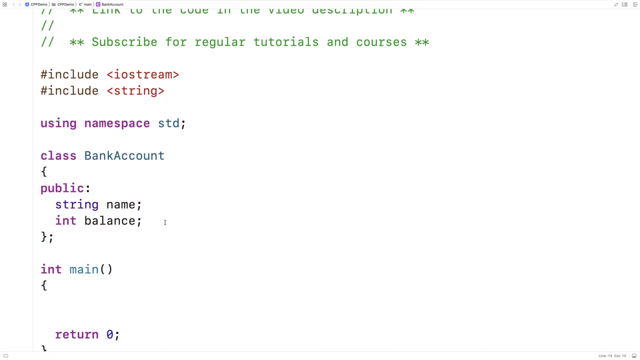 means that these members are accessible from outside of this class here. So what does this mean, now that we have this class of type bank account? What this means is that we can create what are called bank account objects, And those bank account objects are gonna be instances. 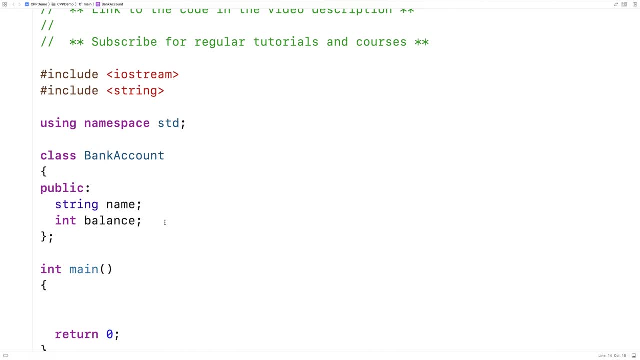 of this class. so the class bank account is basically defining what it means to be a bank account. so if you're a bank account, you're gonna have a name and a balance associated with you. each object is like a specific bank account, so you can have a bank account for you, a bank account for your best. 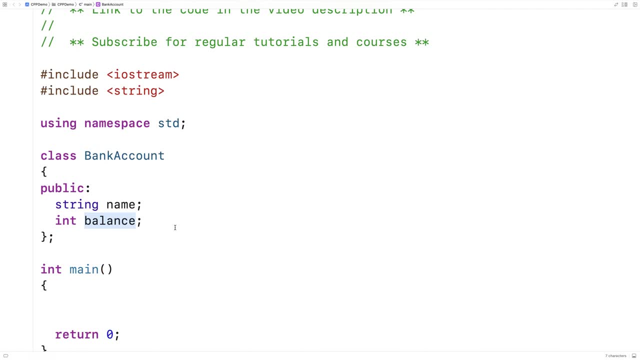 friend, a bank account for somebody, your family and so on. so a class defines what it means to be something like a bank account. objects are going to be the individual instances of that thing, in this case individual bank accounts. so make one here we'll say bank account account one. 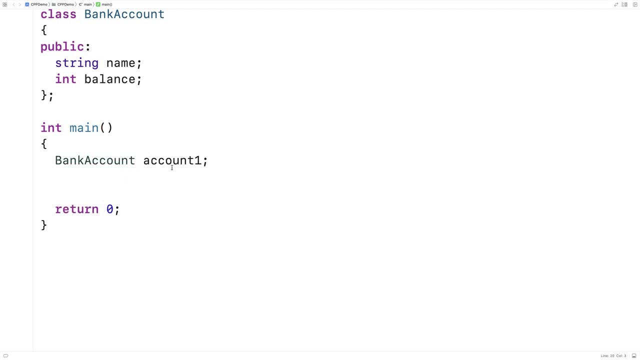 and what this does is. it creates a bank account object and we would say that account one is an instance of the bank account class. it's an object instance. now what we could do is set the name and balance for this specific bank account object by saying account one dot. 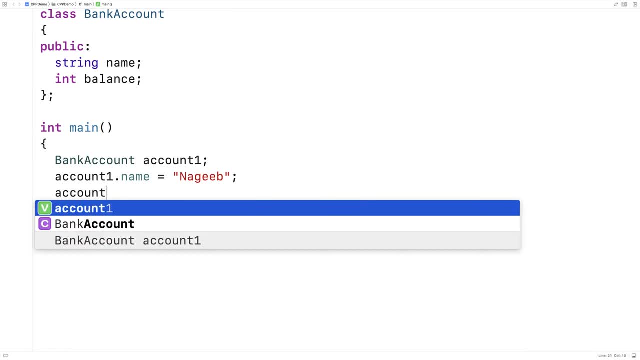 name is equal to Najeeb and account one, dot balance is equal to 3000. so this dot operator here allows us to get at the member variables of our bank account object. so we say dot name, dot balance and we can access those member variables. now, because of this public access modifier, these member variables are available to the main. 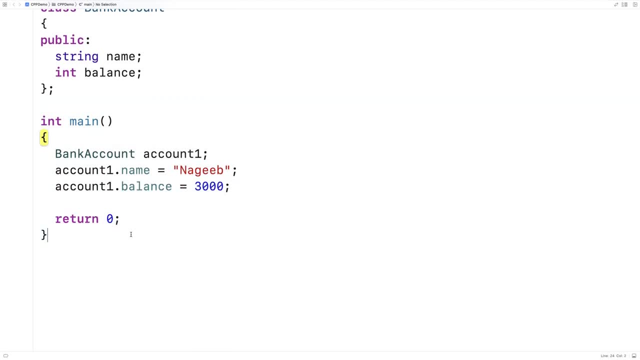 function. there are ways of hiding information associated with an object. we'll talk about those, though, in other videos. we could also print out this data so we could say: see out account one dot name has account. one dot balance dollars and then we'll say endel. so if we save and run this, we're going to get that Najeeb has. 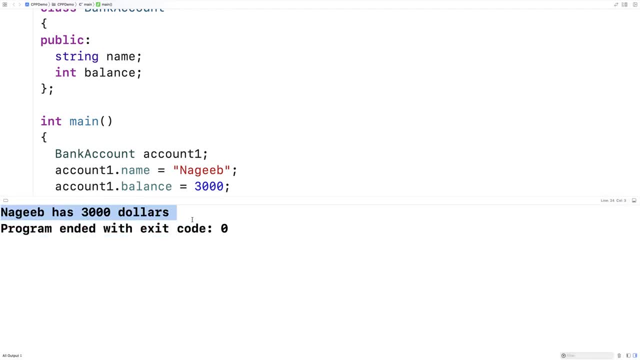 three thousand dollars and that's what we get here. now we can create more than one instance, more than one object for a class. so I could say bank account account two, and this bank account object can have totally different information than account one, because it's a different object, it's a different. 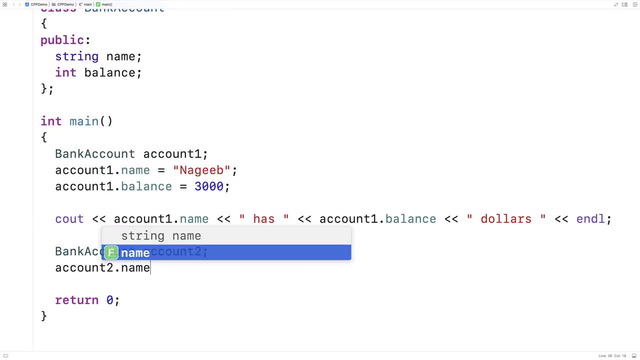 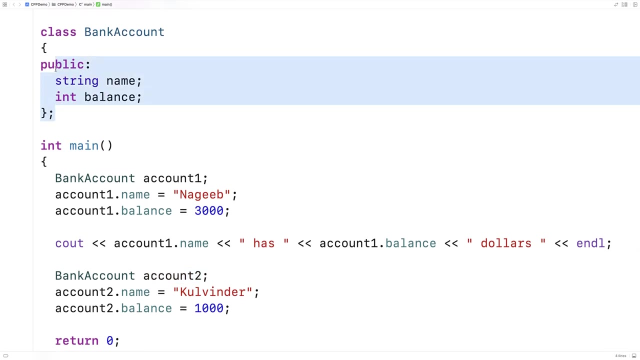 bank account. so we'll say here: account two- dot name is equal to Colvinder. account two dot balance is equal to 1000.. and this account two object is another instance of this bank account class. so if bank account is like a blueprint, we can think of each one of these. 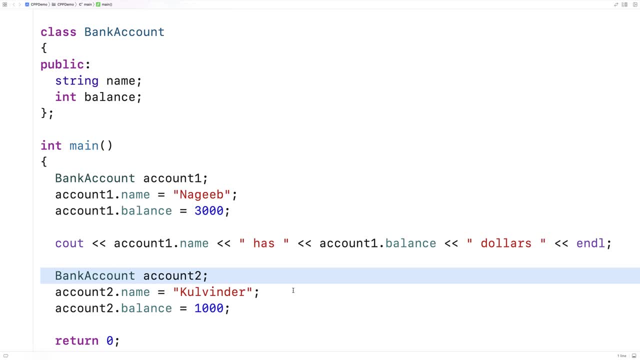 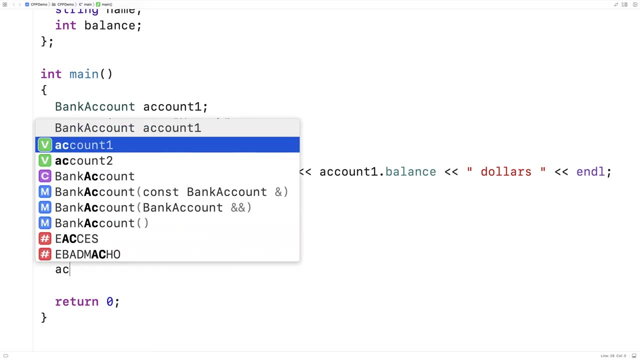 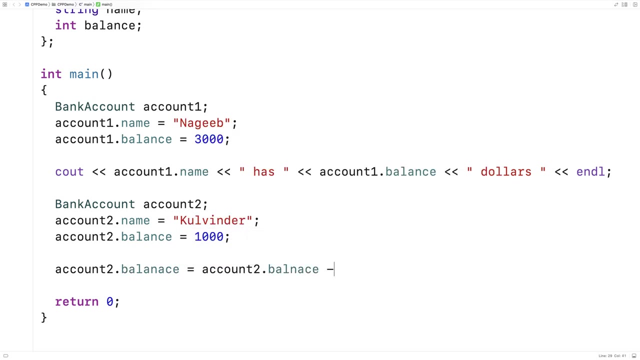 as the house that was built from that blueprint. we could also manipulate the member variables as well, so we could say here: account two dot balance is equal to account two dot balance minus 100.. maybe to perform a withdraw operation with this data and we could output the account balance before. 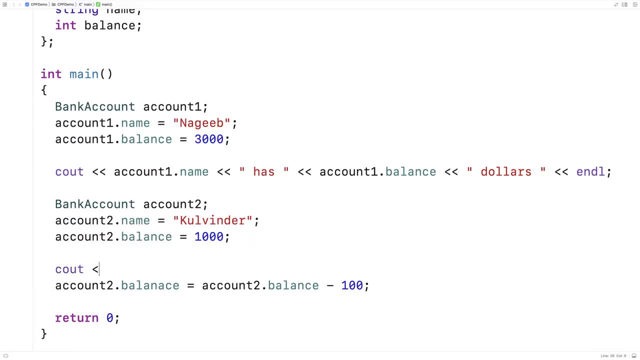 and after this withdraws. so we could say: cout, account two dot name has, and we'll say account two dot balance, and then dollars and then endel, and we'll just copy this and we'll paste it after we've done the withdraw, so we save and run this. 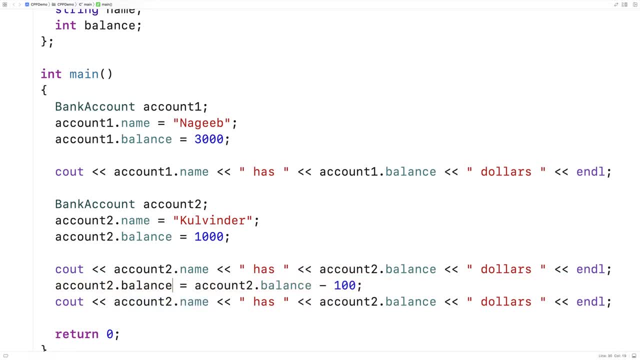 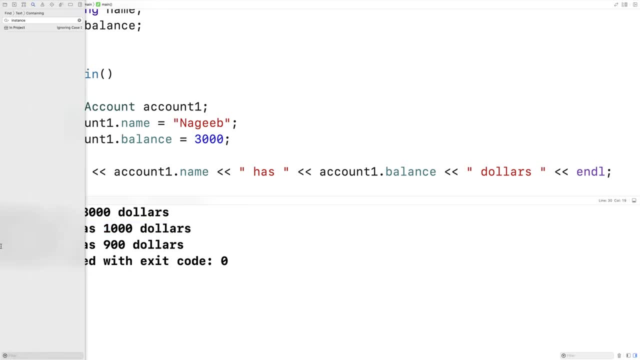 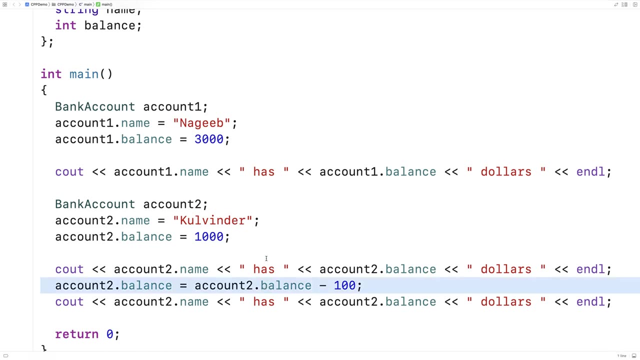 we'll now get that. Colvinder had a thousand, followed by Colvinder has 900.. and we get: Colvinder has one thousand dollars and Colvinder has nine hundred dollars. so what we really have here is an operation, a withdraw operation, that's working with the. 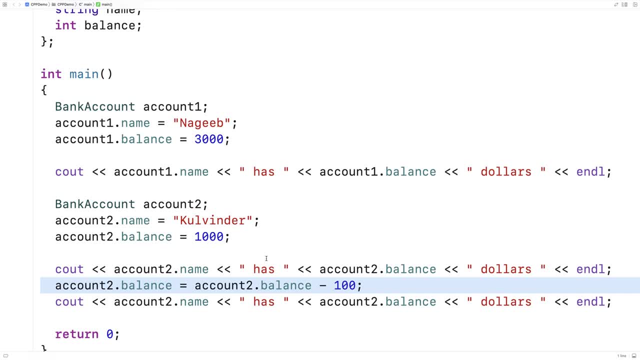 balance member variable of this object. one of the things that's really important about object-oriented programming is that, in addition to grouping together the data that's related, we're also going to group together the related functionalities that work with that data. What we can define are member functions and the member functions can work with our member. 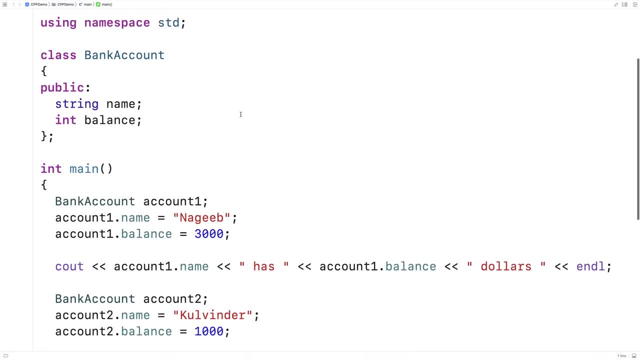 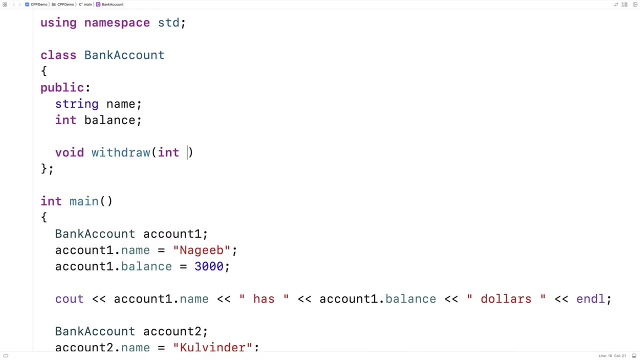 variables. So, for example, we can make a withdraw function. We'll say void, withdraw int amount. So the function is going to accept an amount as an argument and the function is called withdraw. We'll withdraw that amount from the balance. so we'll say balance is equal to balance minus. 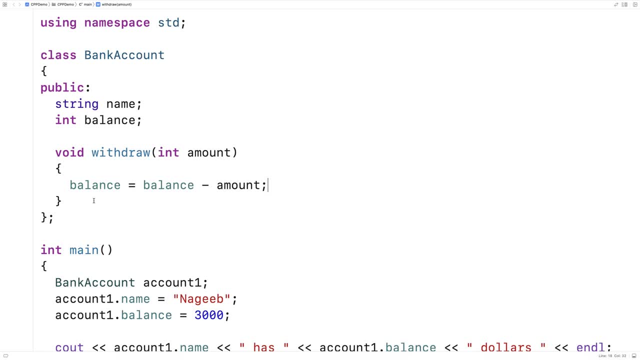 the amount. So our member functions can directly access and work with our member variables, in this case balance, And we're going to subtract the amount from the balance To get the new balance after doing a withdraw. We can call our member functions using the dot notation. 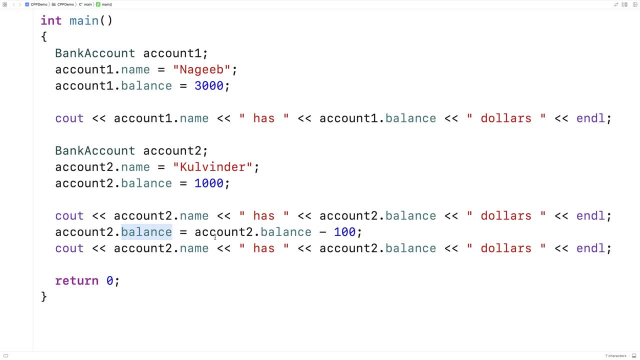 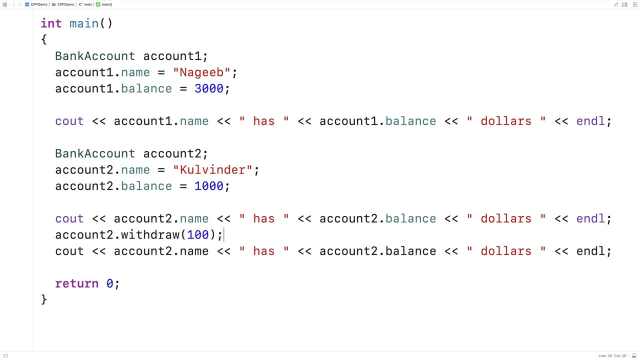 So instead of saying here account2.balance is equal to account2.balance minus 100, we can call that function, We'll say account2.withdraw 100, and if we save and run this, we'll actually get the exact same results as before. 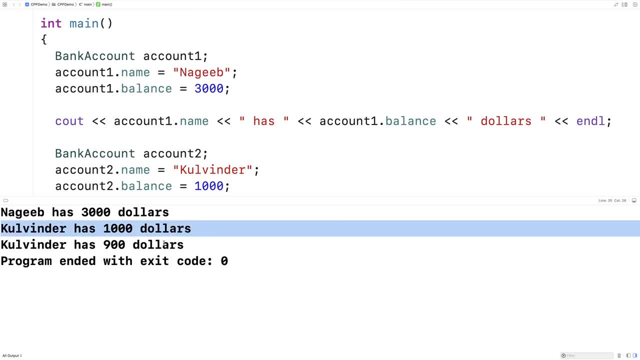 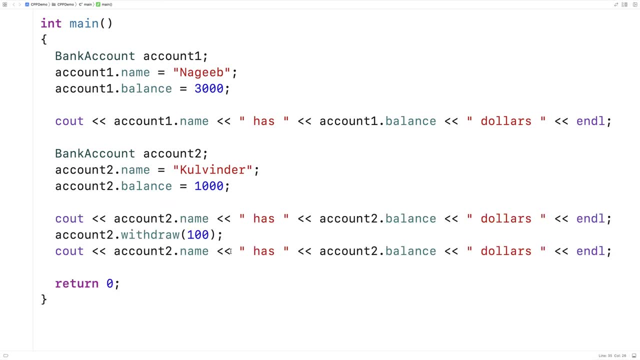 With Colvinder initially having an account balance of 1,000, followed by 900.. After the withdraw, We could also define a member function for this print operation. We basically have a print operation here where we're saying accountname has this balance.